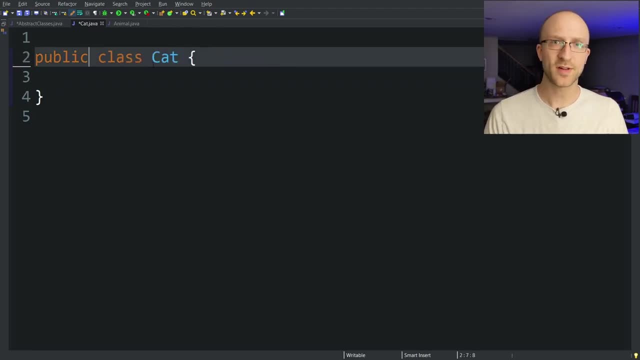 use an abstract class. Let's change this cat class back into a regular class And instead of just being a standalone class, let's say it extended a class called animal And let's say the animal class had a couple of fields like int, age and string name It. 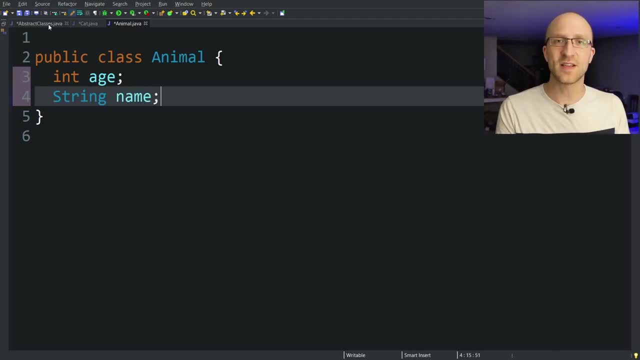 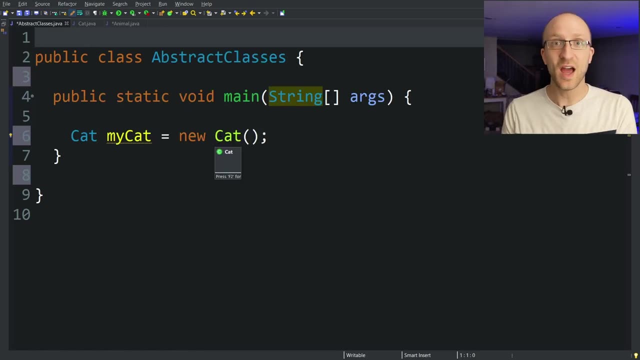 totally makes sense that you could have an animal class that would have subclasses of actual animals like cat, dog, horse, whatever. And it makes sense that you could create objects of those subclasses, Like you could create a cat object. But what doesn't make a whole lot of sense is creating 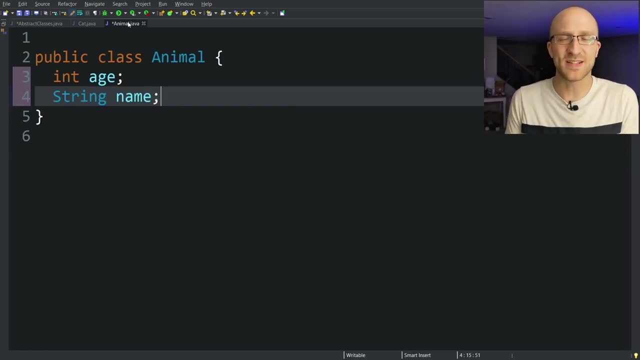 an animal object. You know it's just kind of weird. What kind of animal is it? So you might want a parent class like animal, so that your subclasses can share some fields like age name and maybe some methods that you write But you might not want to be able to create. 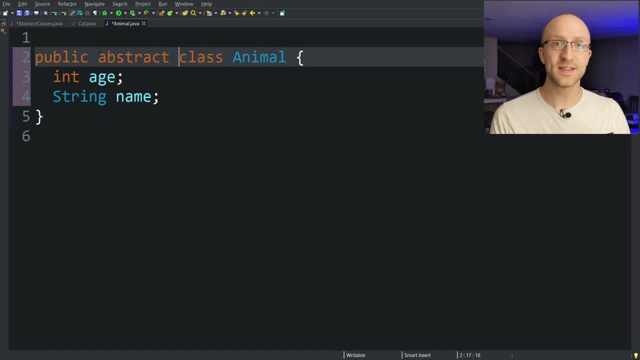 objects of this animal class. All you have to do is make this class abstract. So an abstract class is a class you can't instantiate, but you can absolutely make subclasses of an abstract class that can be instantiated. Now what about abstract methods? In any of your abstract classes you can choose to have abstract methods. Let's say we had a method. 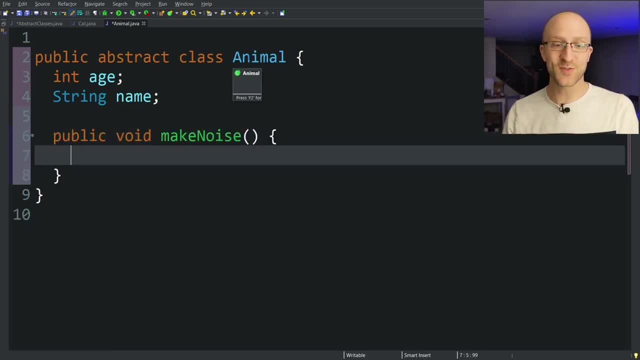 like public void, make noise. Now, of course it makes sense for an animal to be able to make noise, but each individual animal is going to make noise in its own way. A cat's going to meow, a dog is going to bark, So because of that it might not make a whole lot of sense to actually implement. 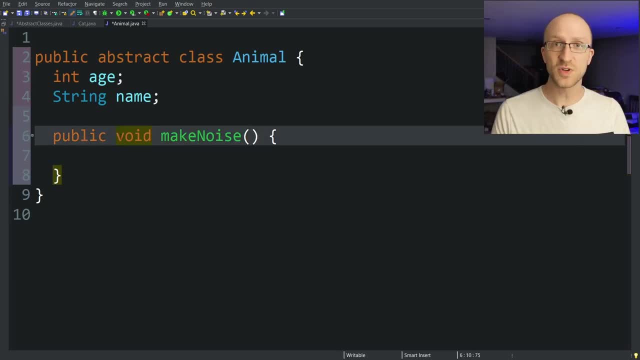 this method make noise here In your abstract animal class. what you can do is make this method an abstract method. When you make a method abstract, you don't specify a body for the method. All you do is declare it and then end it with a semicolon. But then in all the child classes of your abstract class you have to. 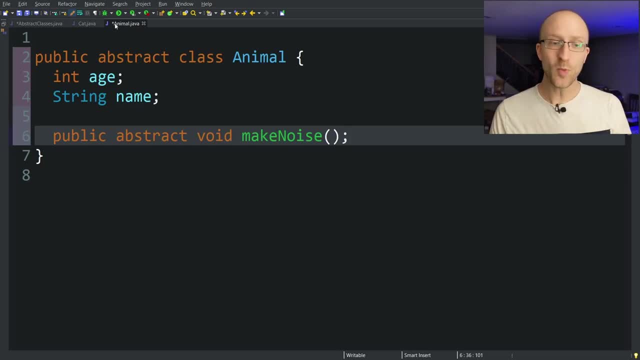 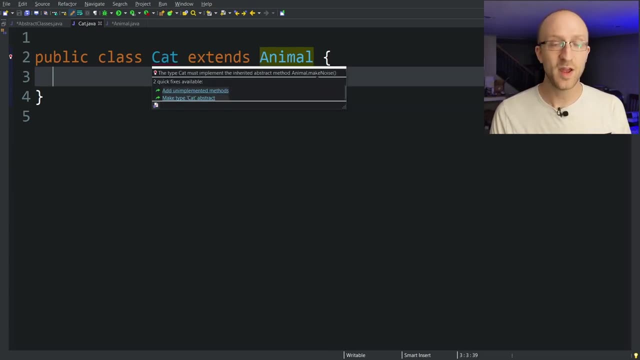 actually create an implementation of this make noise method. So if we go back over to our cat class now, we can see that it's giving us an error, that the type cat must implement the inherited abstract method make noise. So of course we can write it all out, but we can also just use Eclipse's. 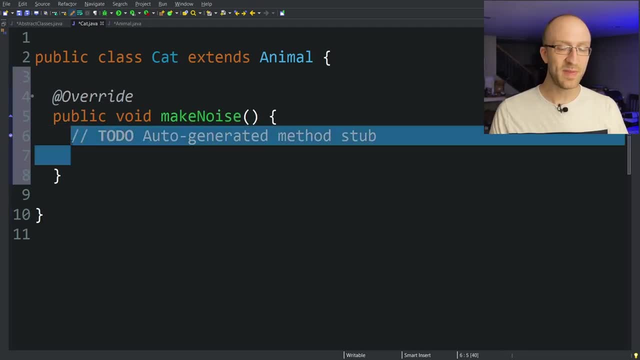 method to add the unimplemented method. But now this cat class can implement this make noise method however we want Print out meow. So because this animal class declares an abstract method- make noise, any child class of this animal class has to provide its own make noise implementation. 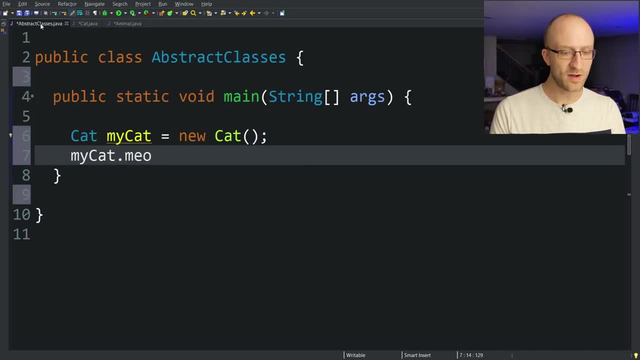 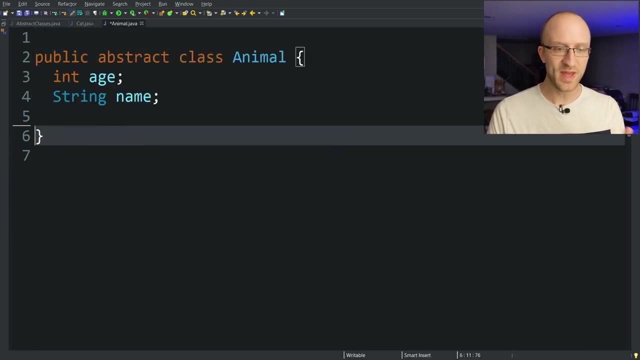 So now back in our main method. we could take my cat and call meow, And if we run our program we can see that it says meow. Now of course we could in our animal class, you know, get rid of this abstract method and in our cat class just declare a make noise method that says meow, And we 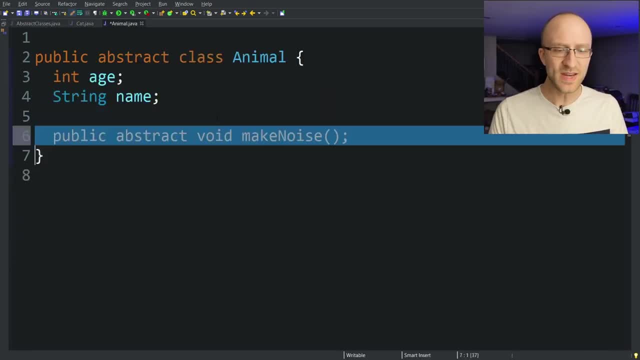 go back and run our program again, it still says meow. So why do we need this abstract method? What do we want that for? What the abstract class does as a whole is kind of enforce and organize exactly what every subclass of animal has to have. So this animal class is saying: hey, if you want to create a 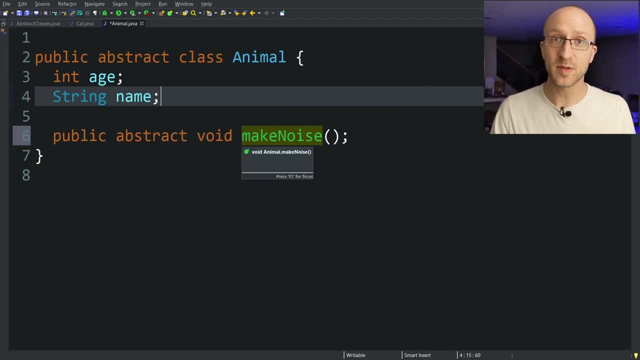 new type of animal. it's going to have an age, it's going to have a name and it has to be able to make noise. Every type of animal might make noise in completely different ways, but this makes sure that every single animal type is able to make noise. As a side note, though, in your abstract, 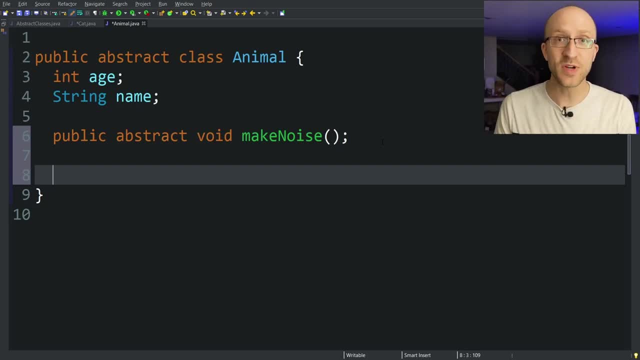 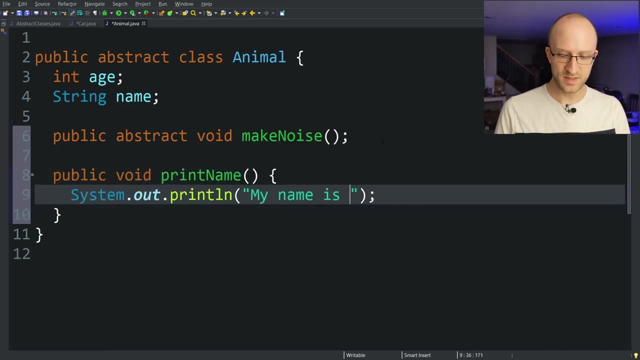 class. you don't necessarily have to be abstract. You can create actual concrete implemented methods in your abstract classes So you could have like public void print name just prints my name is name. So now every subclass of animal will also have this print name method available to it. but since 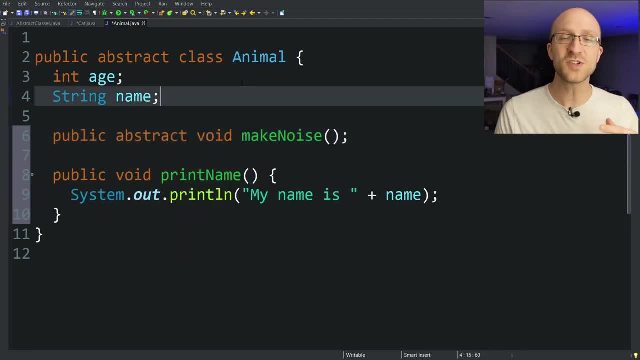 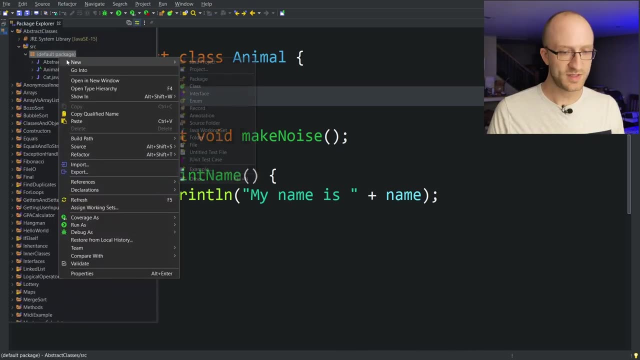 it's not abstract. they don't need to implement it themselves. They can just use the implementation. that's here The question a lot of people have- and what's actually also a big interview question- is: what's the difference between an abstract class and an interface? Let's say we had an interface. 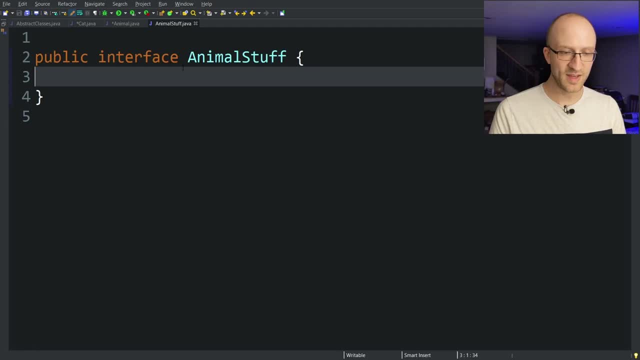 called like stuff. Here in an interface we could say: how about public void poop? Just like every animal might make noise in different ways, every animal is probably also going to poop in different ways. In interfaces. you don't need an abstract keyword in your methods. Every method in an interface is: 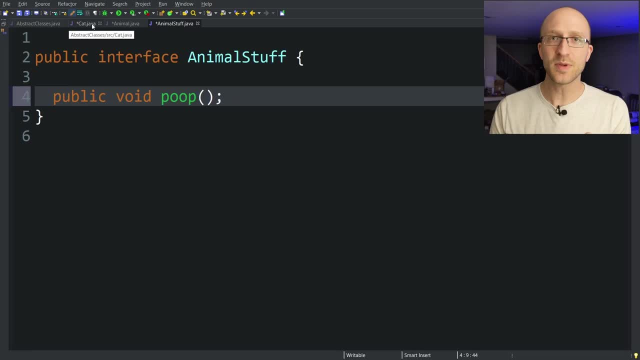 assumed to be abstract, so you don't need this keyword. As you probably know, if you want to implement an interface, so all you have to do is, instead of extending another class, you just say implements the interface, which is animal stuff. And now that we implement this animal stuff, 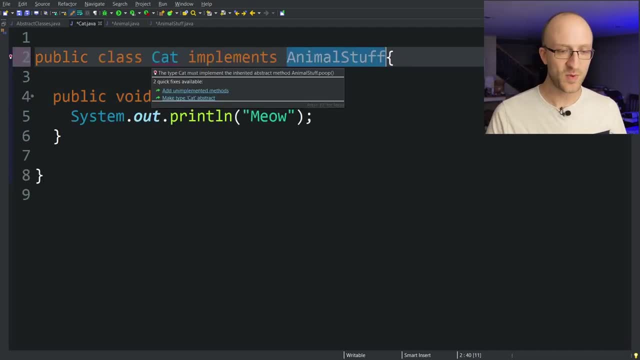 interface, we have to implement the interface. So now that we have this animal stuff interface, we have to implement this poop method. You see, right now we get an error that says the type cat must implement the inherited abstract method poop. We can just click the suggestion here to add.